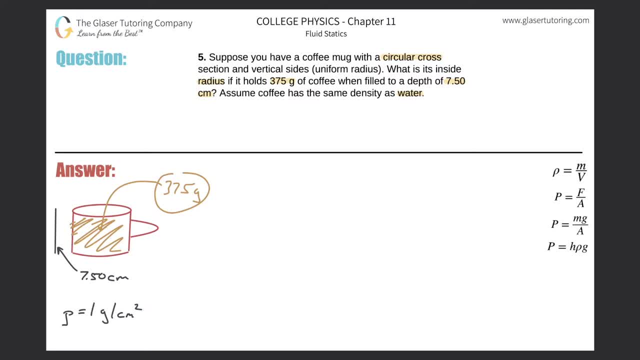 two, It's not per centimeter squared, It's per centimeter cubed. So just seeing if you're paying attention, of course. So what we do know here is, again to get back on track- we do know the weight of such water and we do know the density of such water. 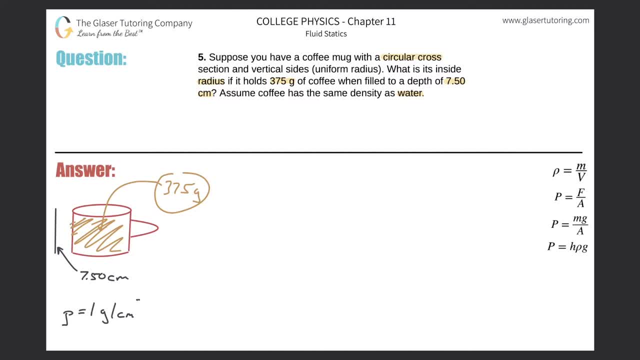 And therefore I can easily find the volume of such water okay, by simply using the density formula. over here I noticed the units are consistent between my mass unit there and my mass and my density, So I can just simply use this formula that density is equal to. 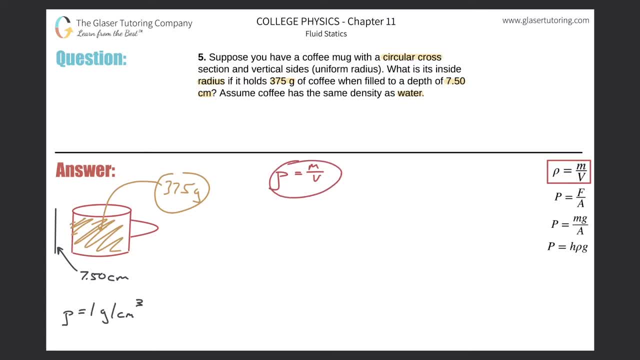 mass over volume, And what I can do is substitute or solve this thing for volume. right, I can say that V is then equal to the mass which we know, divided by then the density, which we also know. So I'm going to leave this alone for right. 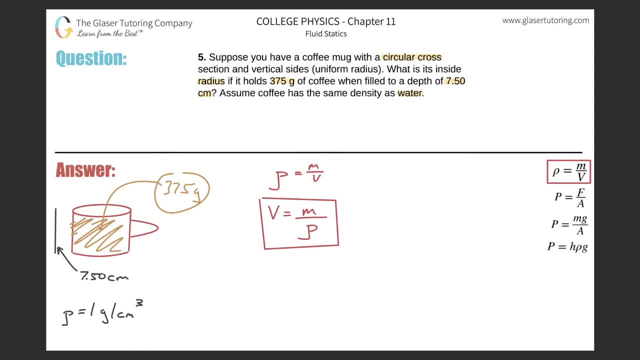 now, because I'm just going to do a bunch of substitutions. Now, if I know the volume, somehow I need to find now the radius. So in my picture here's the radius, okay, So I need to somehow find this R value. So what you're thinking is how in the world 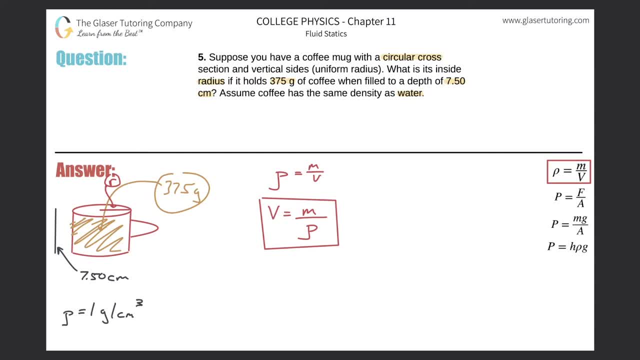 is volume, then connected to radius. Oh, wait a minute. What's the nature of this object? Oh, it's a basic cylinder, right? So we know that the volume of a cylinder is actually a value of the mass, of the mass. So what we're going to do is we're going to 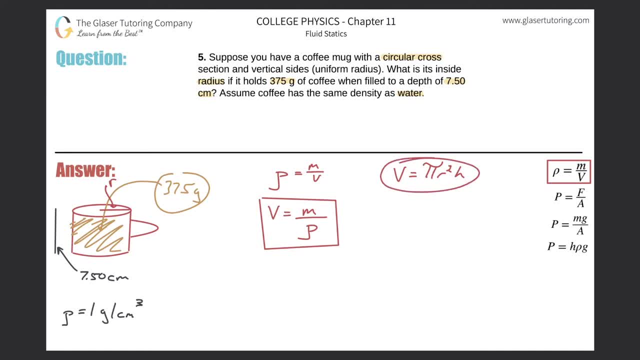 solve this thing for R, and then we're going to add a new value for that. So it's going to be R squared over pi, R squared H. Oh, my goodness, and look at this right. This basically tells us: if we solve this thing for R, okay, divide out the pi and H from both sides, so we get R squared is. 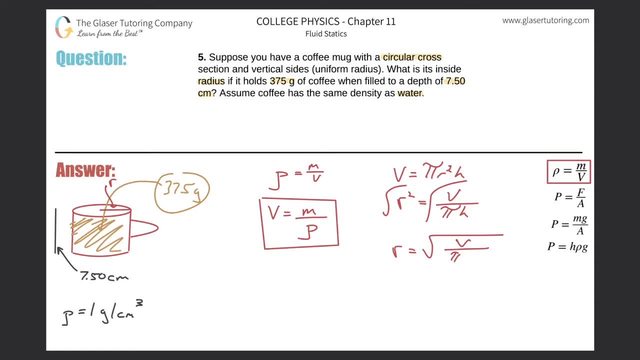 equal to V over pi H. And now take the square root of both sides right to find R by itself, And what this tells us is that we need to know the volume and the height. And we do know the height value. they told us: okay, now we could convert everything here to meters if we wanted. all right, 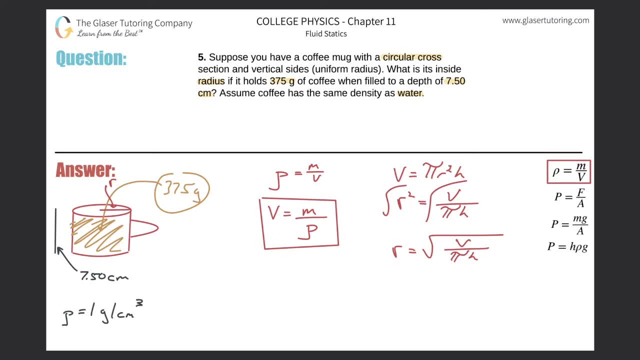 we really don't need to. as long as the, as long as the distance value here- okay, the centimeter correlates with the cubic distance value here and the mass value there correlates and is the same as the mass value there. we don't have to do any such conversions. all right, so now, all i'm going to do